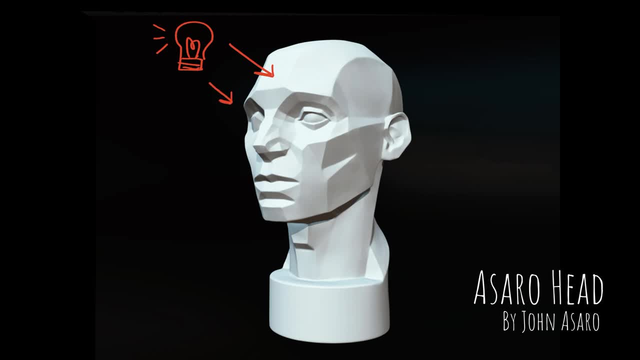 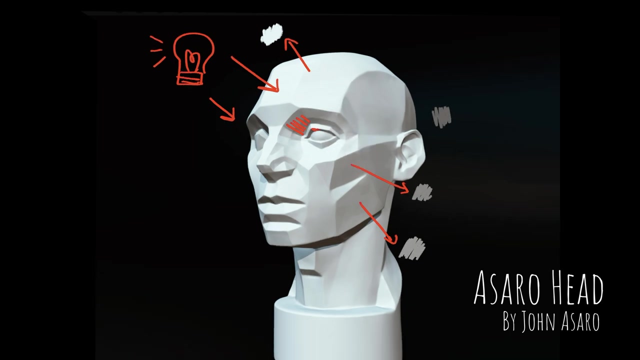 while on the ones in shadow we are going to have darker values and the head is all made with the same material. so there's no difference in this case and in fact, we will have a value that goes towards white on the upper planes and we can have slightly darker values on the planes that are not. 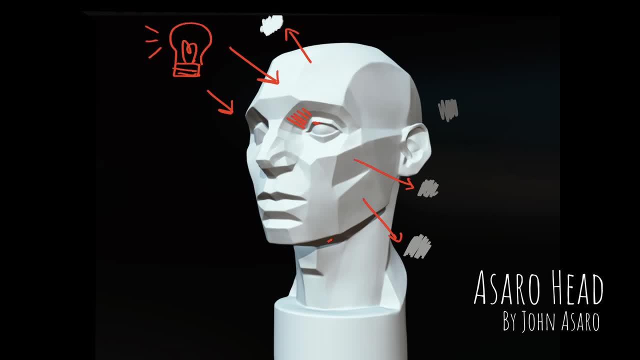 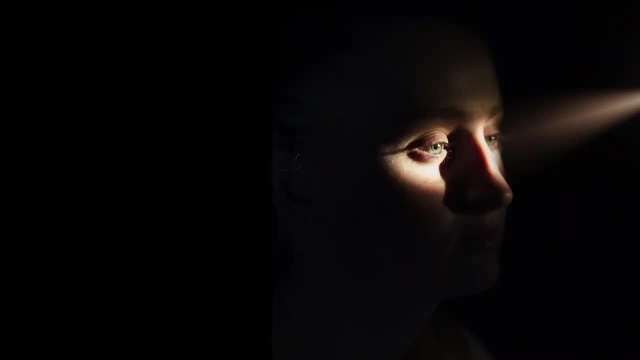 facing the light, so the ones in shadow. The azaro head is a great example and you can find this model on sketchfab and I'll include a link in the description. So the TLDR for this is everything we can see- is light and it's tanked to values. All we have to do. 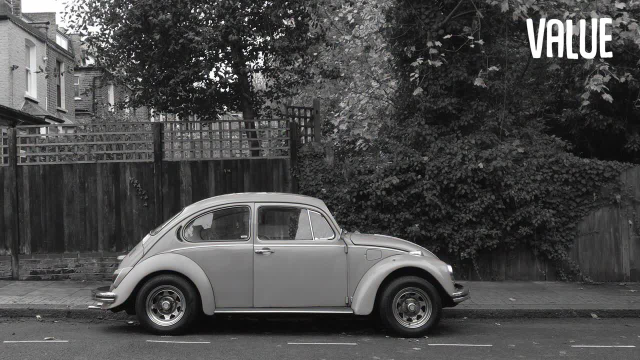 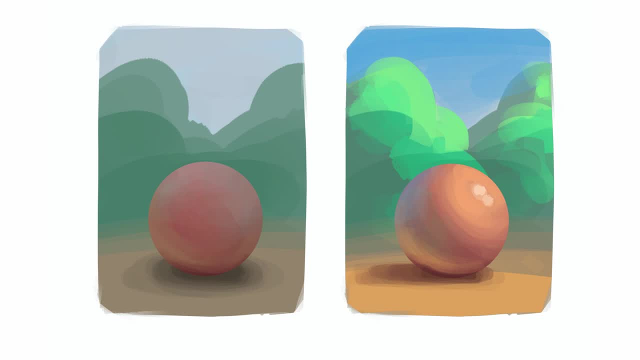 to find the values of an image is to turn it grayscale, basically like with this picture, and because grayscales remove the colors, we can have an objective view of the values that we are seeing. so how the light interacts with each material, how the light interacts with each surface. 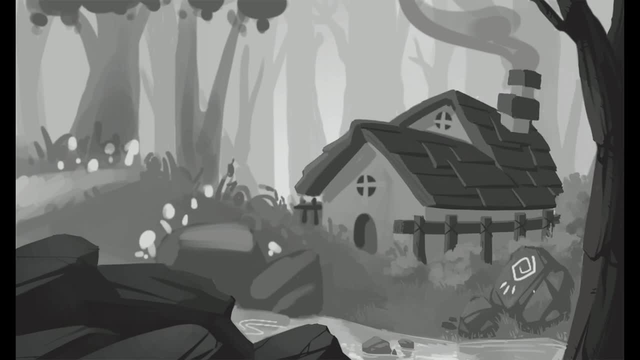 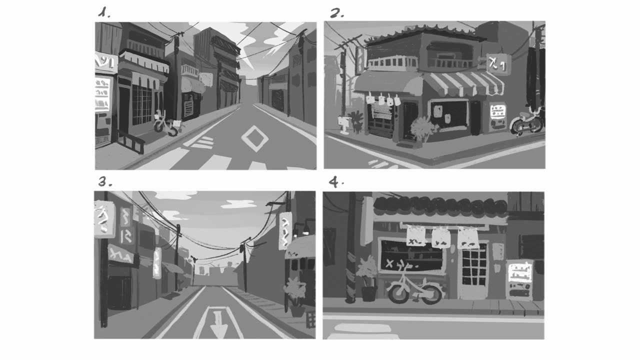 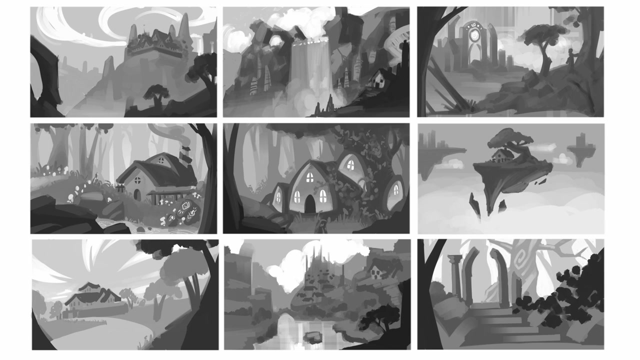 Using values and grayscales is a great method for focusing on light behavior only. I usually use this technique for thumbnails and for sketching and for when I want to focus on idea and composition for a painting, when I don't want to add color in the equation, in order to keep things simple and not over complicated. 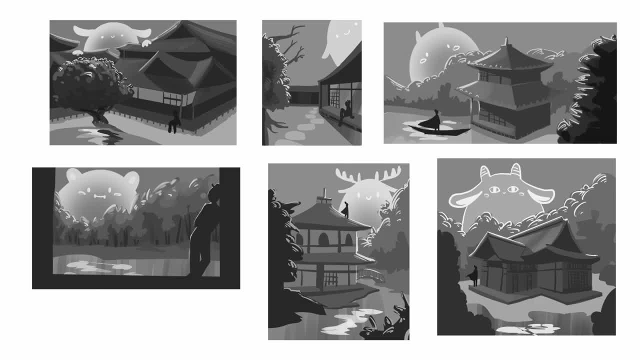 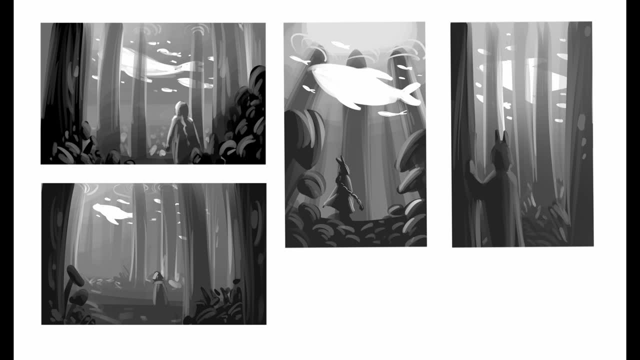 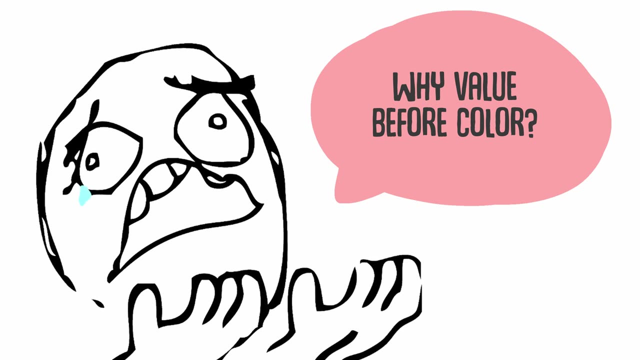 Like in these examples. these are thumbnails that I usually do to prepare for a painting and, as you can see here I only focus on composition and light behavior pretty much Now. as you can see, value is really important, but why is it so important and why is important to master value before color? 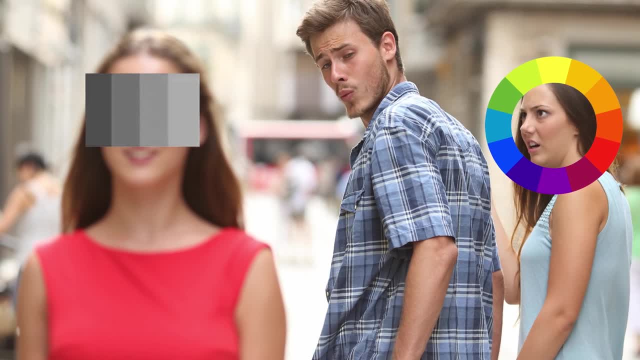 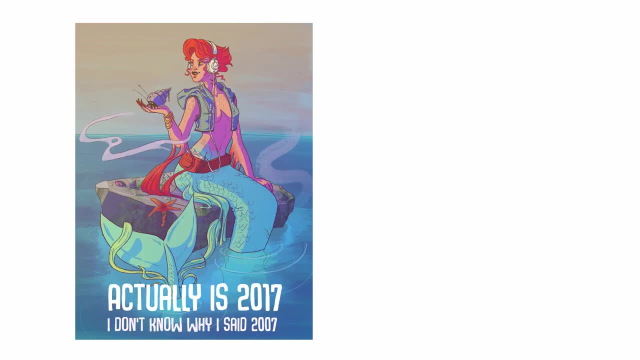 Well, the reason is simple: nice colors would never save bad values, because value is the foundation of the image. Here we have a couple of examples. this is a painting that I made in late 2007, while the mermaid on the right is a painting I did this year, and the difference in 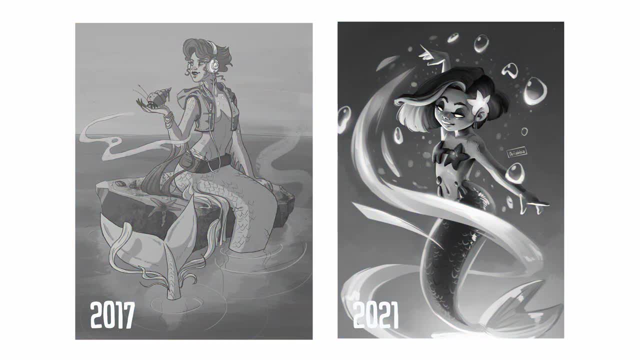 values is incredible. as soon as I turn them grayscale, you can notice that in the image on the left, the values are all over the place, While in the image on the right, on the mermaid, you can see that I clearly have an area of focus, and 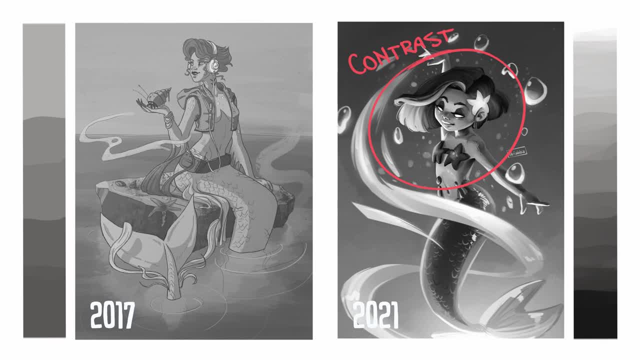 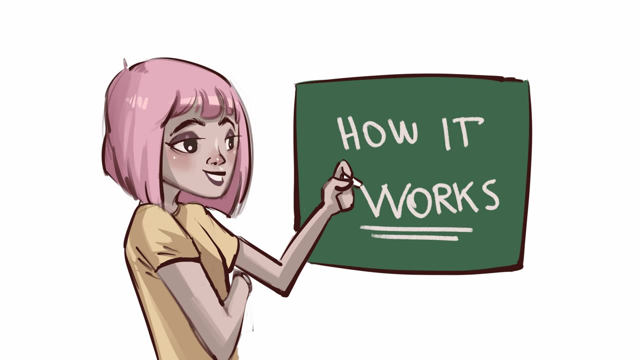 all the contrast and the focus goes on the mermaid in the right places, while the background is just pretty much flat. values and, by result, the image on the right is much more readable than the image on the left. Now let me explain how value and color works in an image. 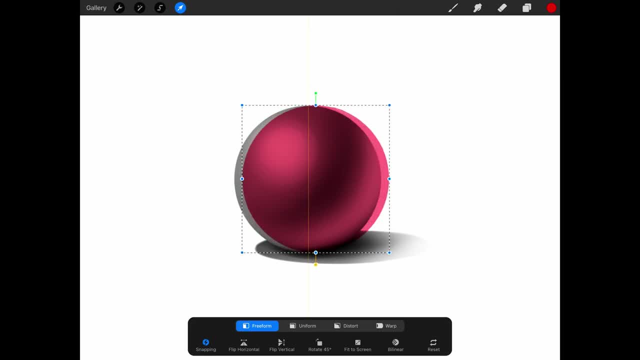 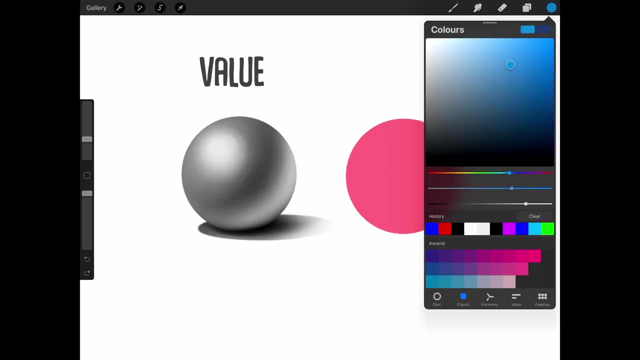 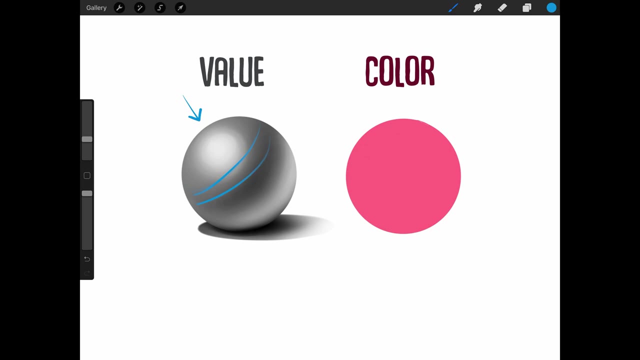 You can clearly see in this red sphere that I have both color and value, but as soon as I separate the them and I keep the value on the left and the color on the right, it's really evident that what remains in value is the whole 3d shape of the sphere, while the color element gives me back. 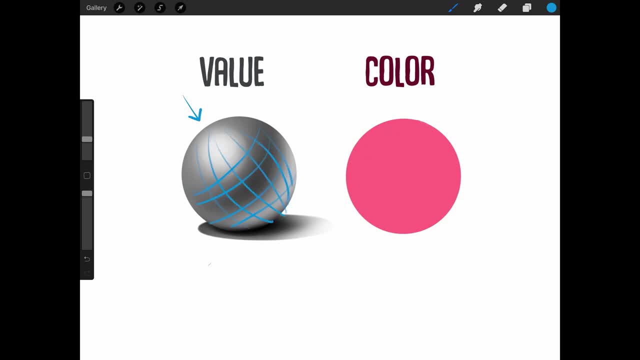 just a 2d image. This is the difference in readability between value and color. We can see color as the cherry on top of our composition. this doesn't mean that color is not important, but it means that all the readability of the masses, that it's comprehensible to the human. 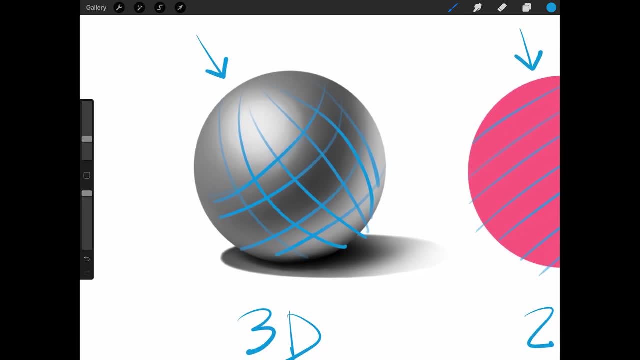 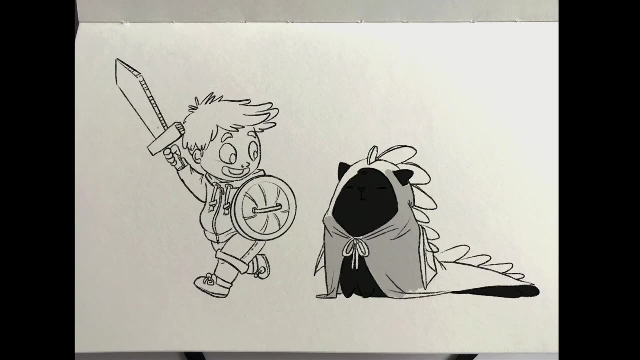 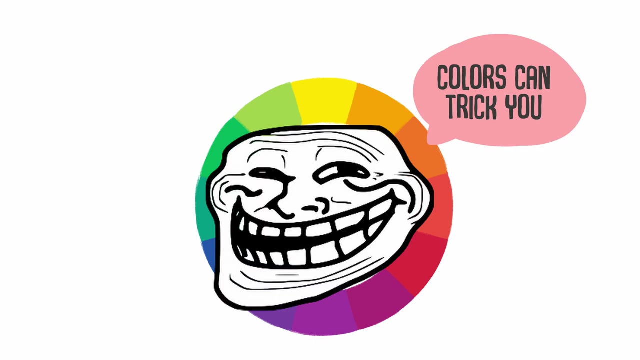 is very important. It's basically only values. So this is why mastering values is really important and it's fundamental to learn before we go on with colors. Another reason why it's often helpful to establish values before color is because color can really trick you. Let me explain why. 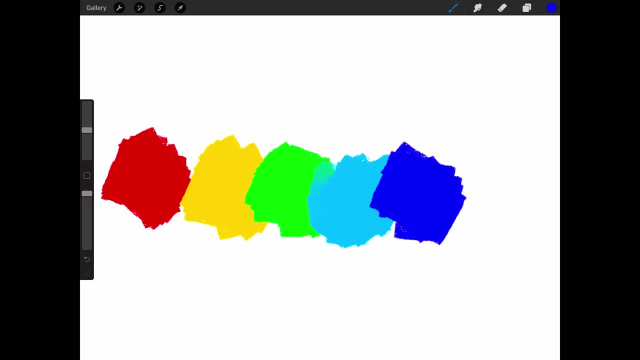 If I pick a series of colors and I pick them all at equal saturation, then I fill a layer with black, can turn them grayscale. You can see that they all translate to different shades of grey, and this is always true. Yellow and the full point of saturation of 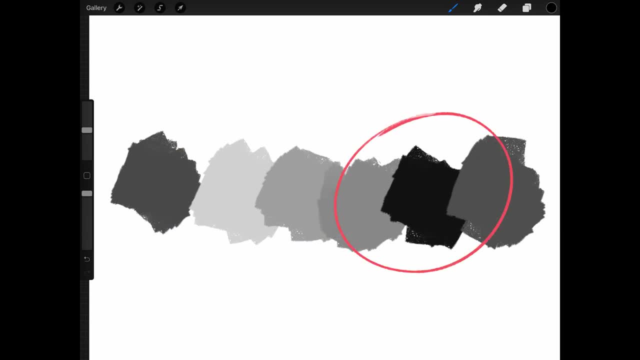 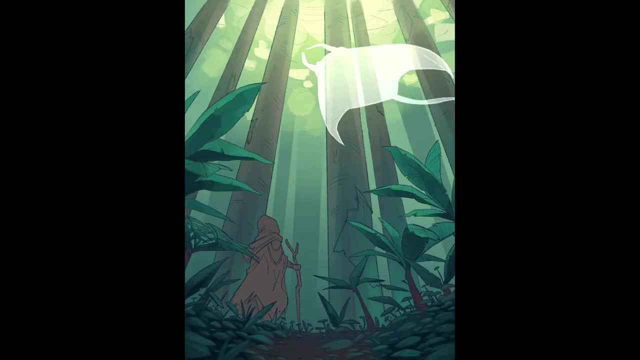 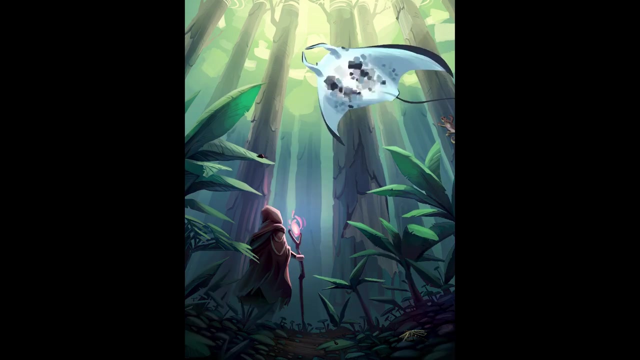 yellow is going to always be lighter than the full point of saturation of blue, for example. So you can imagine that if you are painting directly with colors instead of going through value first, you can very easily lose track of what your values are. Sometimes a difference in colors can give us a full sense of. 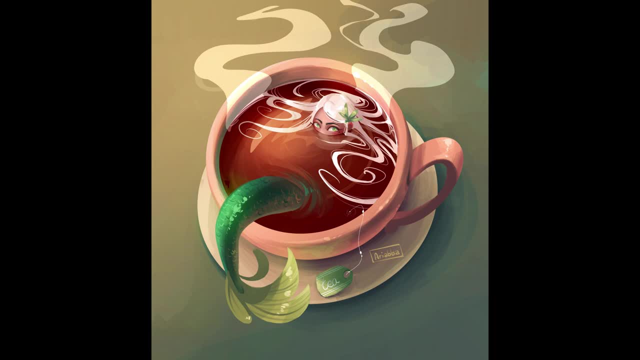 contrast. Let me explain. If we look at this mermaid and we see her for colors, we can see there's clearly a contrast between the T and the tail, because they are two complementary colors close to each other. But if we turn it grayscale. 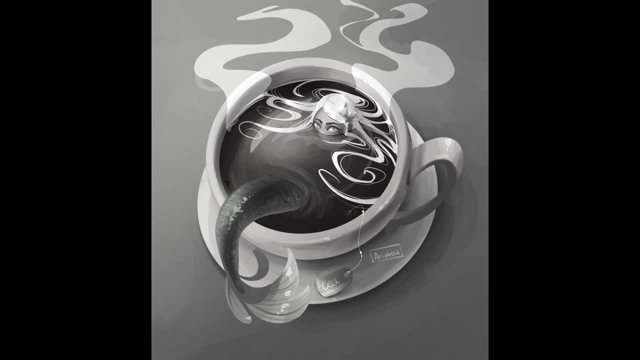 we can see that actually, the T value and the tail value are pretty much the same. If we were to do things correctly, either the tail or the T should have a different value in order to contrast the images. This way, we can change more and drive more attention towards the subject. 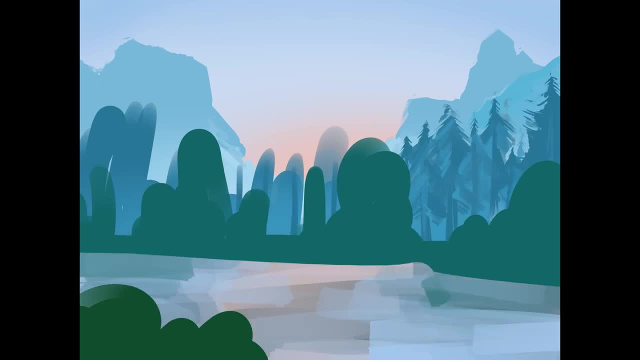 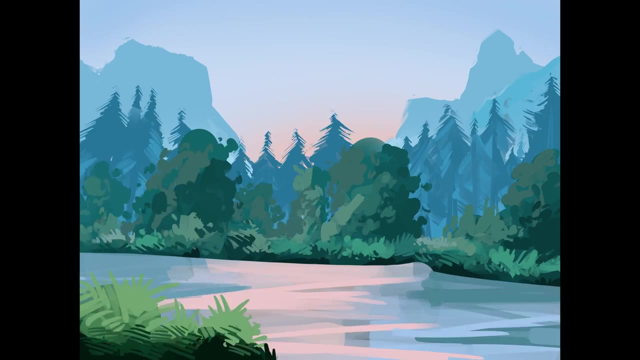 Now I'm not saying you should start every painting with values first, because I don't do that either, But sometimes, if you want to concentrate on composition first and on light behavior, it can be pretty useful and it can end up simplifying your process. 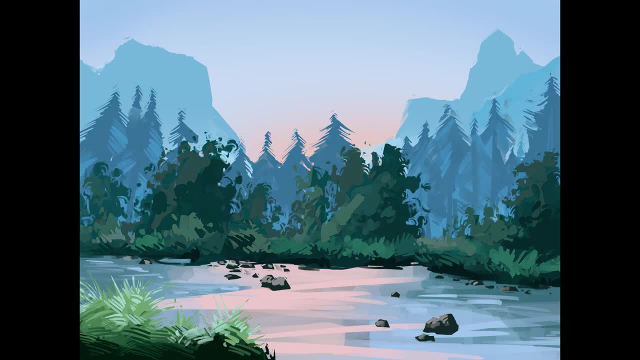 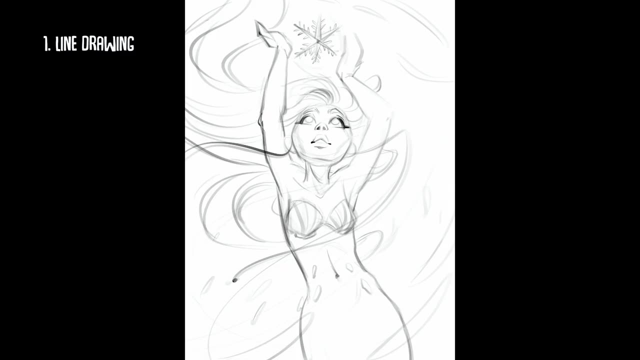 Now, to explain this point, I'm going to show you two examples: One where I start with values and the other one where I start with colors. When I start with values, I can focus on composition with values. Now, when I start with values, I can focus on composition with values. I can focus on composition with values and I can focus on composition with colors. Now, when I start with values, I can focus on composition with colors. I can focus on composition with values and I can focus on composition with colors. Now, when I start with values, I can focus on composition with values. 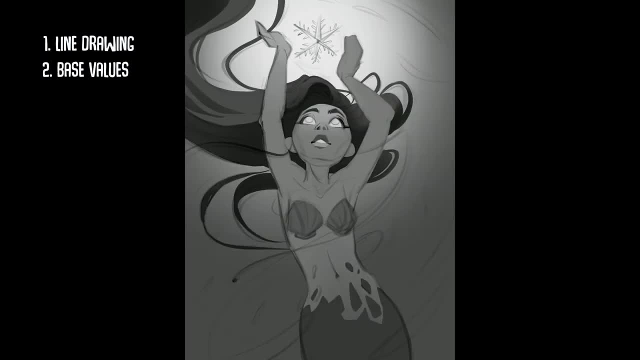 Now, when I start with values, I can focus on composition with values. Now, when I start with values, I can focus on composition with values. I can focus on composition with values and I can focus on composition with colors. Now, when I start with values, I can focus on composition with values. 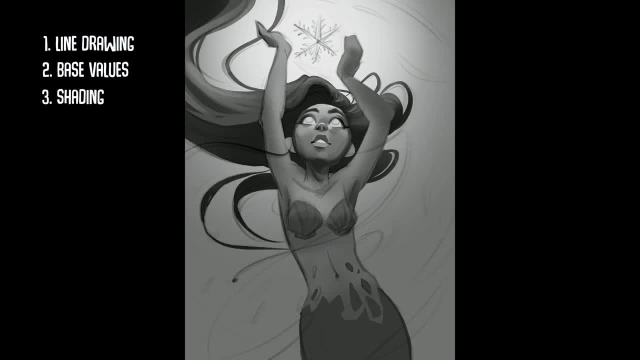 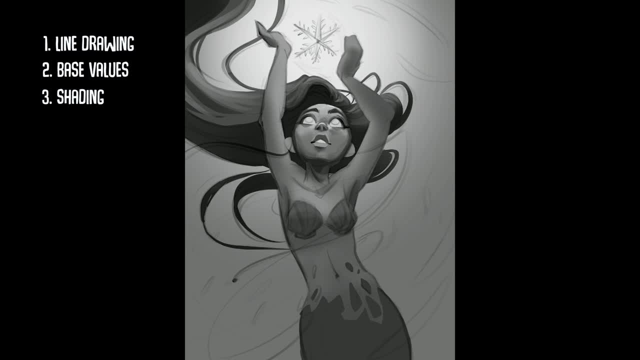 Now, when I start with values, I can focus on composition with values. Now, when I start with values, I can focus on composition with values, adjust some superficial things later with the colors. This is a much simpler process and allows me to focus on the important stuff first. At the end, the 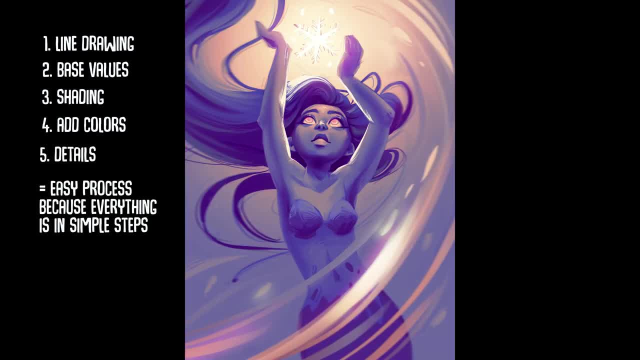 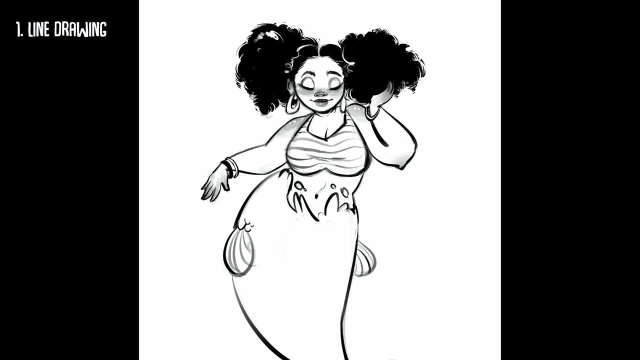 colors are just the cherry on top and I can just noodle with the details later. When I start with colors instead, my priorities shift a little bit. I worry about the palette first and I put the flat colors down. Then I worry about the. 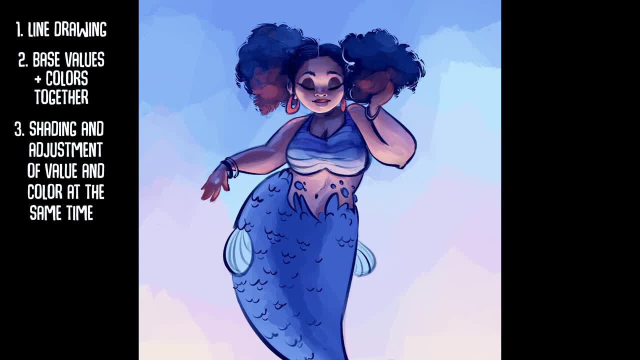 values and shading properly, and I adjust everything as I go forward with the painting. This means constantly checking that everything works together, and it can be really complicated because there are many things to keep in check all at once. So while I worry about the color combinations and the palette, I also 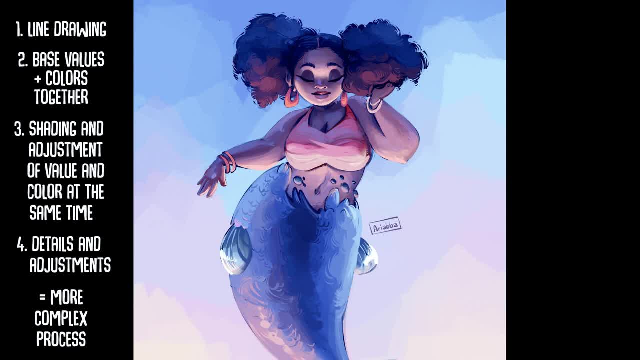 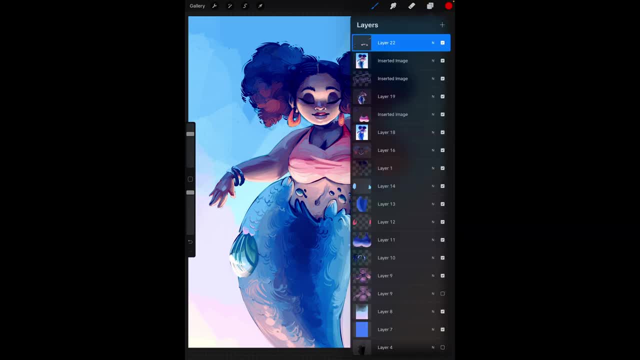 worry about shading properly, light, behavior and composition. Now, if you don't know it, a good trick for keeping your values in check when you are painting directly with colors is this one: You can make a new layer on the very top, fill it with black, and then you can use the blending mode. 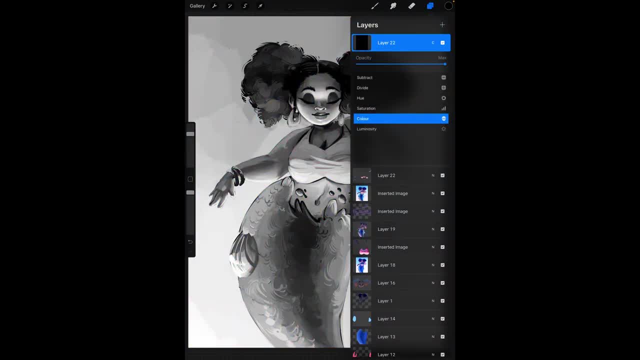 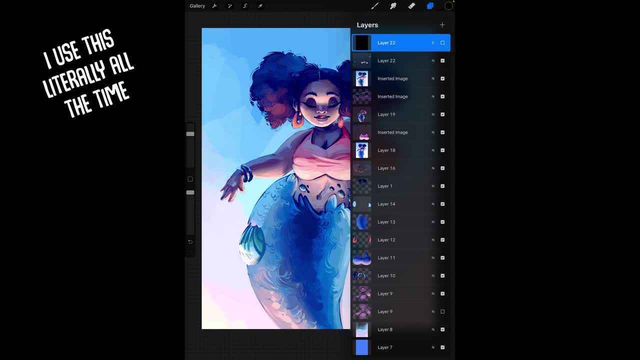 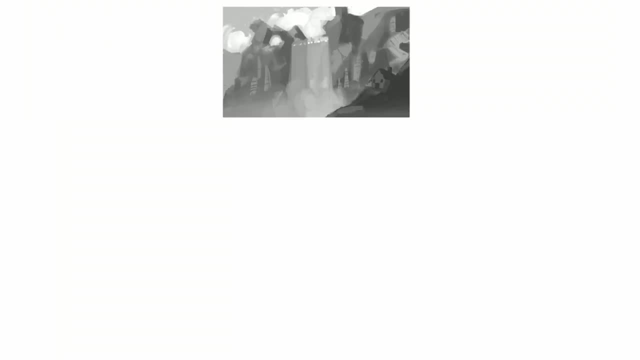 painting in colors, but you can constantly check the accuracy of your values and adjust everything as you go. Now you can see that proceeding with colors directly can be more powerful, but you should also have a good understanding of values and it can make the process a little bit complicated. 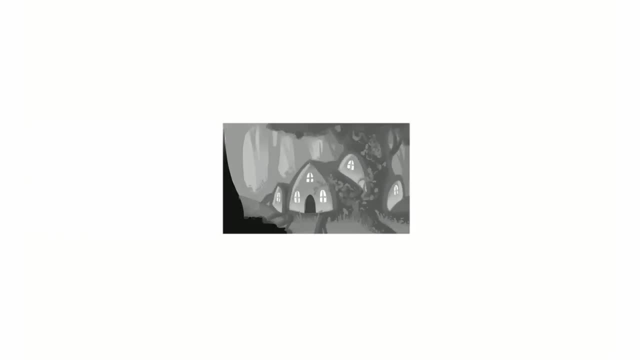 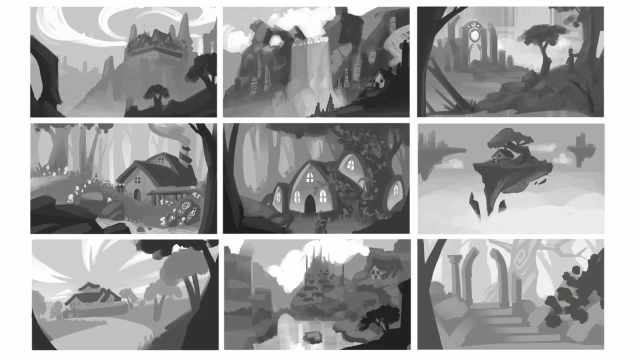 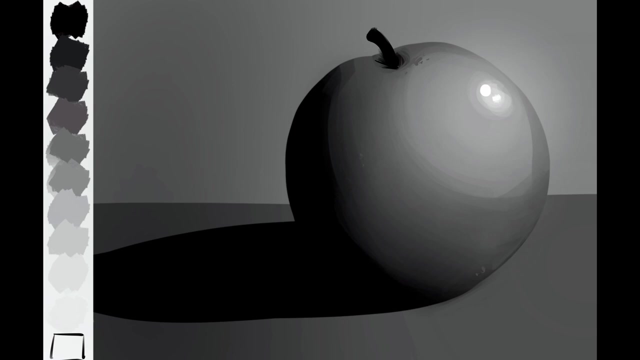 especially if you are a beginner For most complicated paintings. if I really wanted to focus on composition first, I do start with values instead of colors. Now, at the beginning of the video, we saw how light impacts our values, So we can obtain correct values if we start with a certain value and then 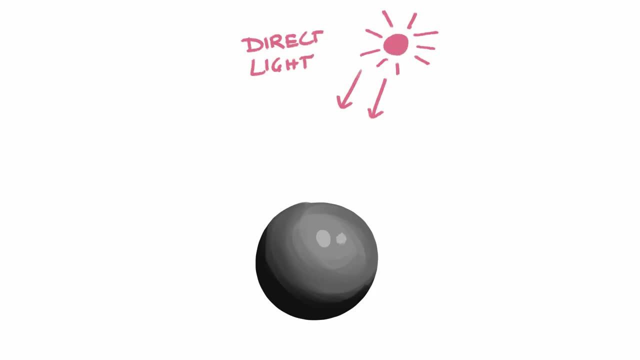 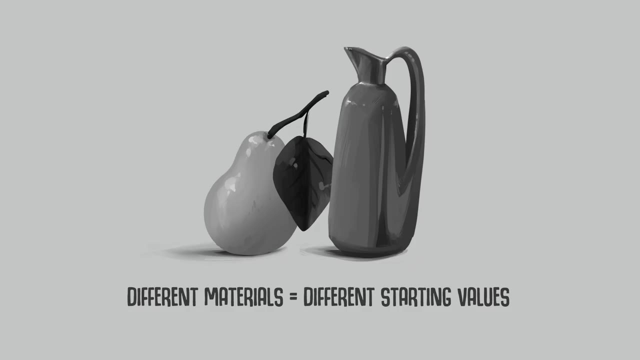 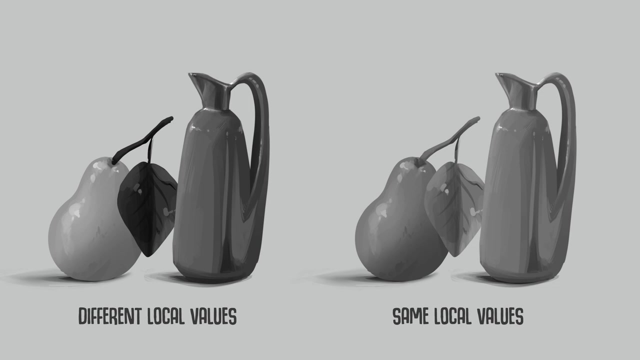 we apply light or shadow, So we shade our object. But what happens in a situation of ambient light? Will all our objects have the same starting value? Well, the answer is no, Because our materials and our surfaces can be different. the local values can be different. A common beginner mistake when 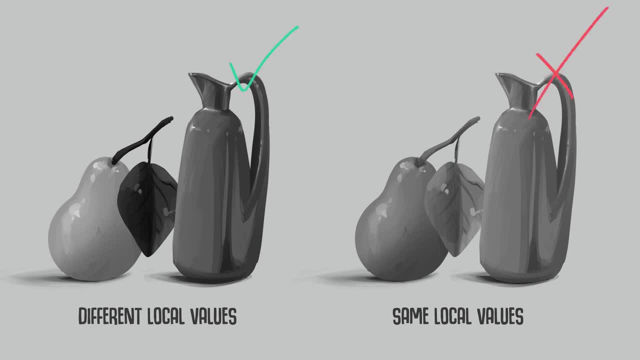 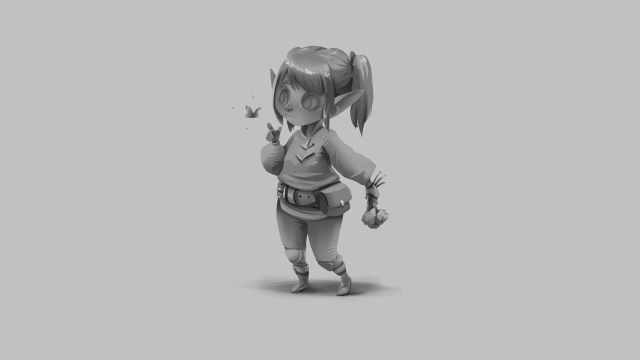 painting in values is not considering local value and paint every object starting with the same local value And it looks like a 3D model without textures. So what happens is that you obtain a model made of the same materials with just ambient occlusion on it. If you don't know what ambient 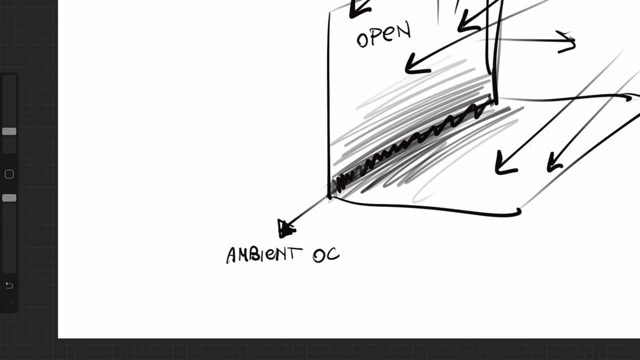 occlusion is. check out this other video where I talk about ambient occlusion and a bunch of other stuff. Now you can see the difference between these two models. One has ambient occlusion and the other has ambient occlusion And the other has ambient occlusion. 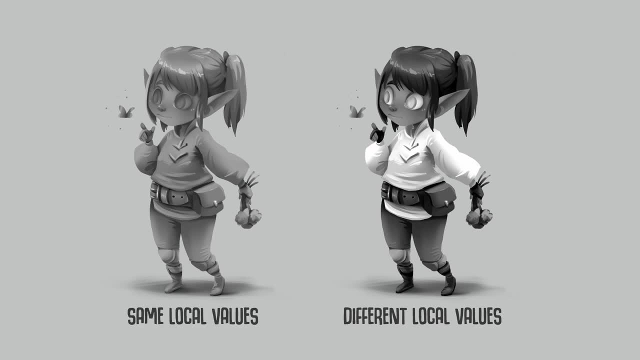 correct local values and the other one has the same local values for everything, And you can clearly see which one of the two looks correct. Now, even if you understand the importance of local values, starting painting with values can be really overwhelming. This is because the human eye 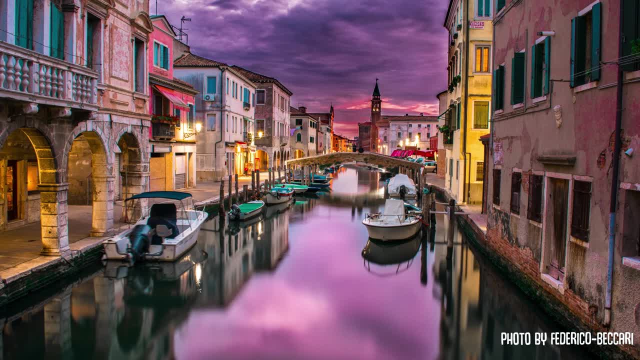 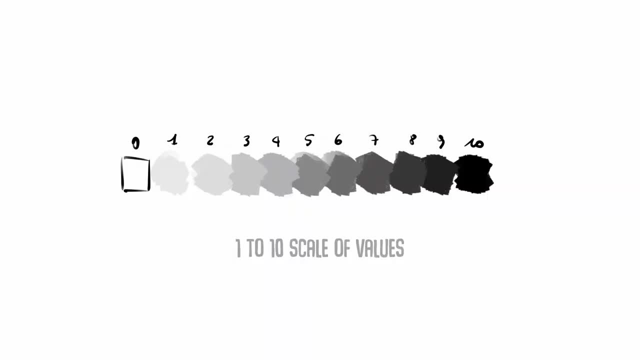 can see billions of values And it's really not realistic that we could use such amount or such range as artists to represent reality. So, in time, artists came up with a way to simplify values and use it in a scale from zero to 10, where we can go from complete white to pure black. This can 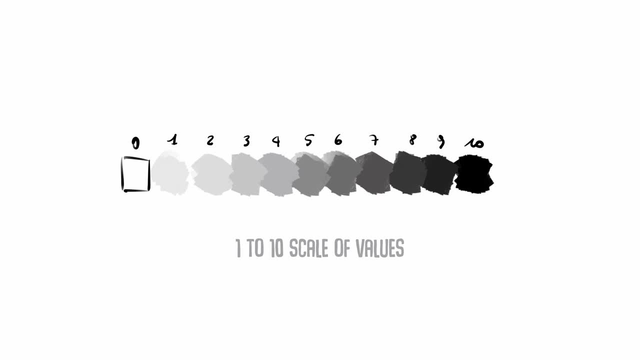 simplify the process pretty much and it can make it more familiar and easy to use. I don't usually recommend to use all 10 values for a painting because, depending on the mood and the subject that you want to represent, it's often better to use just a small range of this, For example. 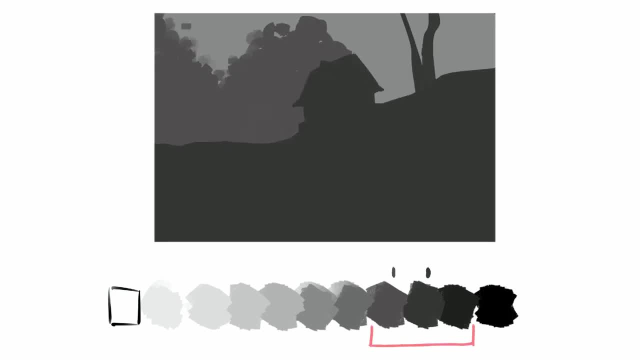 if it's a particularly dark scene, you can use a couple of values towards black and mostly, and just one that goes in the upper middle range. It's better to use a subset of those based on the mood and the atmosphere that we want to convey, Usually as an exercise. 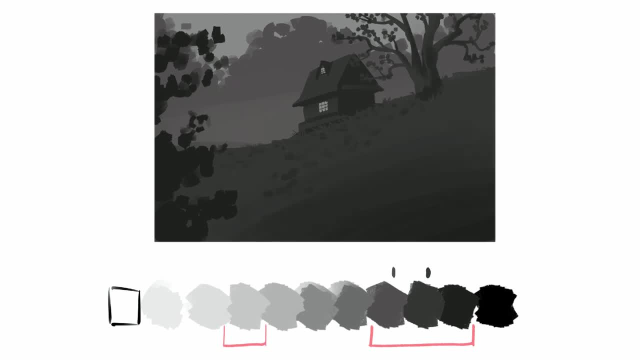 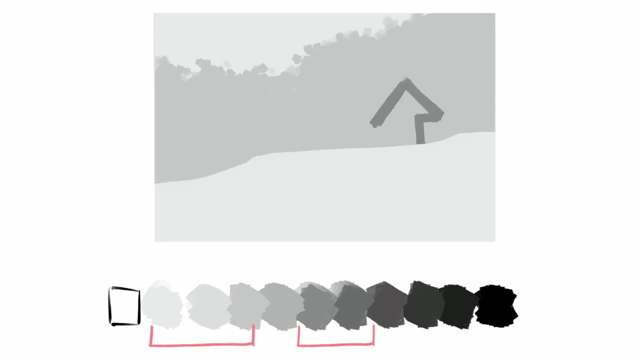 I recommend watching movies and take some still frames from some movies that you want to represent, that have a mood that you like, and try to re-represent this with just three or four different values. I do this as an exercise, sometimes to get in the habit of using values. 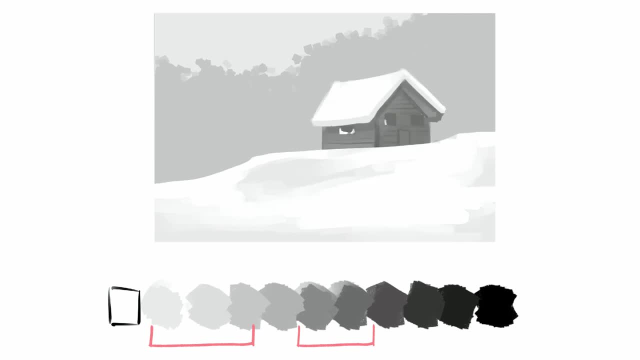 and to get used to it and make them become my comfort zone so that even when I work with colors, I can spot if some values are probably not working properly and if there's no contrast in the area towards the subject that I want to like highlight to the viewer. So, personally, I really recommend. 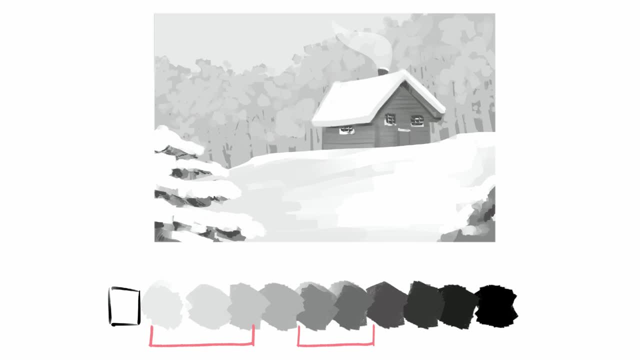 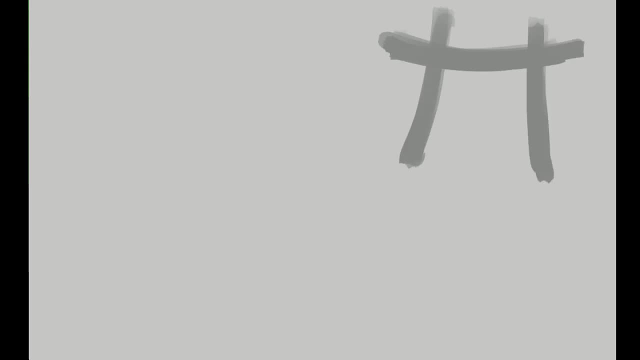 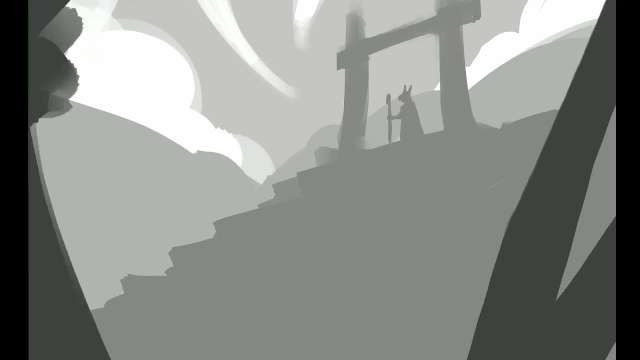 to use this as a frequent exercise to understand values. Now let me show you my process of working with values from scratch. This is a composition I came up with on the fly. I start with pretty much three or four range of values, and my idea is to use the darkest value for elements that are close to the camera. 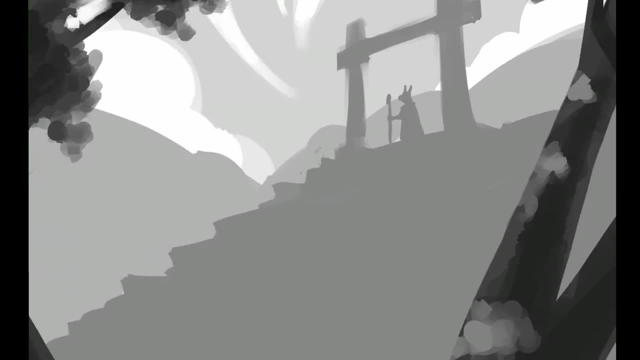 and the farther I go from the camera, the lighter the value is. This is because, basically, when you're looking at a landscape or some very open space, you can clearly see that the further you go, the more atmosphere there is between your eyes and your. 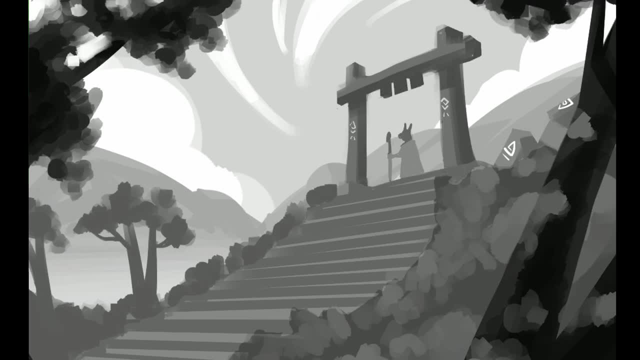 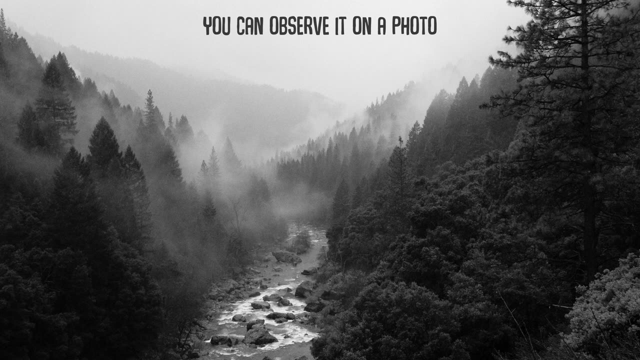 object that you're looking at. So, for this reason, the values are flattening up. If you think about, for example, some landscape that you've seen with mountains in the background, it's very likely that the subjects that you see and the objects that you see 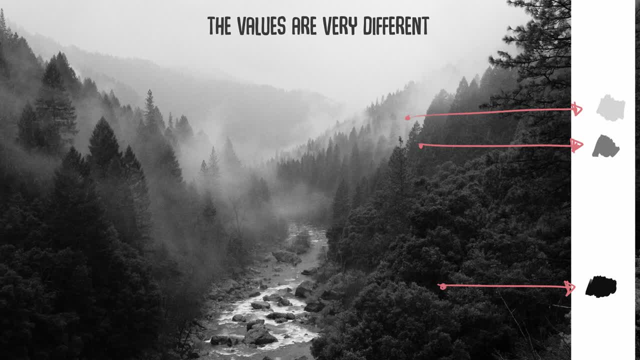 that are close to the camera will have a lot of contrast, because there's little or no air between you and those objects, while the mountains farther away will be usually towards blue or, depending on the weather, but usually with, like, very light or flat values. So this is why I 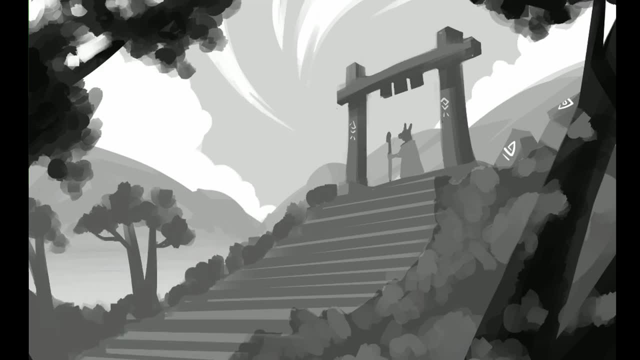 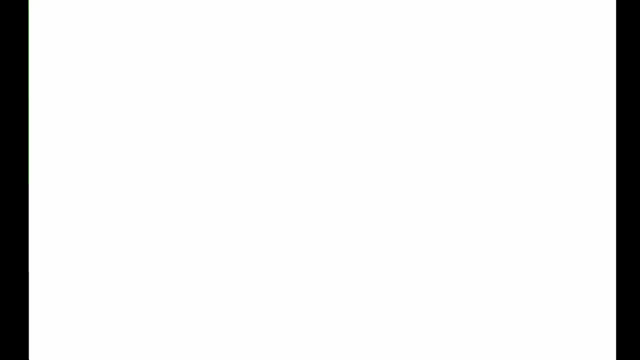 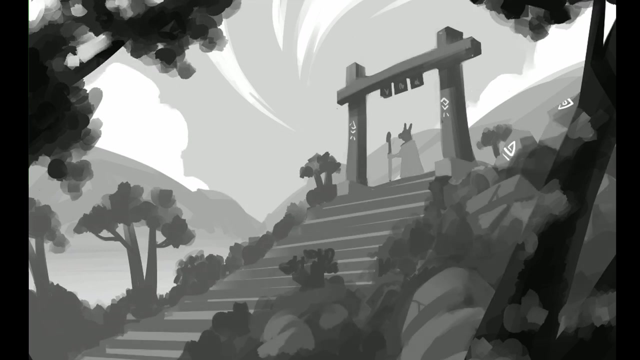 often start with three or four values and I use the darkest one for the closest elements. As I go forward, I try to define the silhouettes of each layer. I keep as much as I can on separate layers based on the silhouette, but I try not to have everything on separate layers because 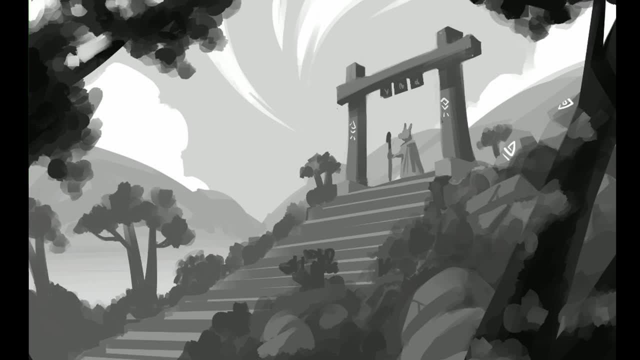 otherwise I will go crazy in no time. I also try to give some indication of light, basically, and try to understand what planes are in shadow. So, for example, in the torii on the top, I can clearly see that there are some parts of the torii that are in shadow, while some other. 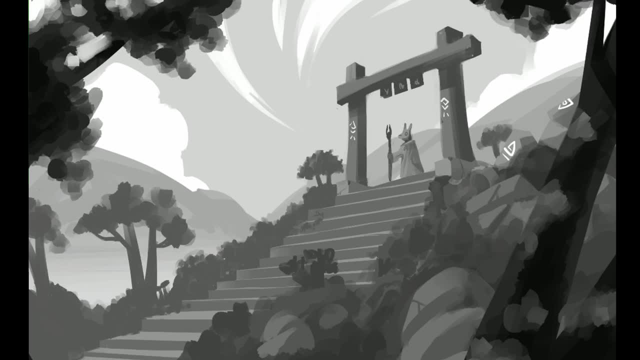 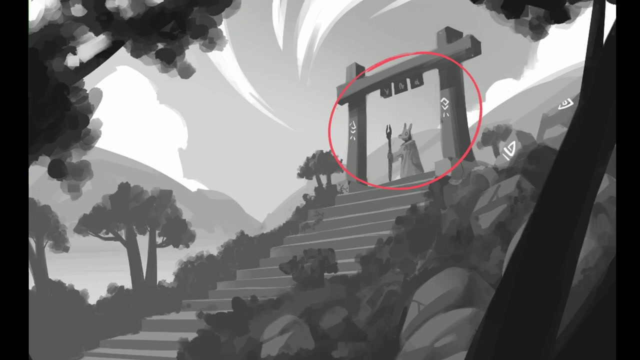 parts are in light, and usually the sky is actually the lightest part of all. Another way to use the difference in values is to try to point the eyes of the viewers towards your subject. So at some point during this process, I decided that my subject at the 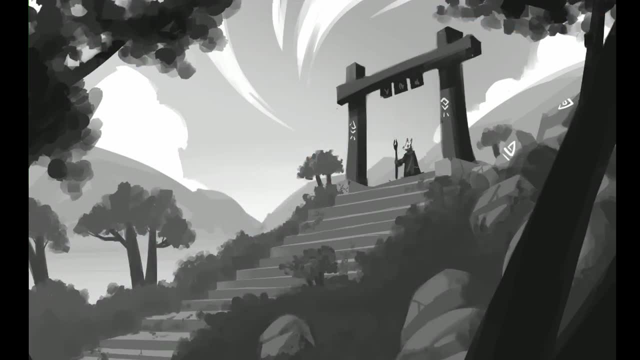 top of the mountain was not visible enough, Probably the torii, the gate on the top, and if you observe the character. I also used the value of the sky and the light that generates from its stuff to create more contrast and this way will catch the eye of the viewer more and will be. 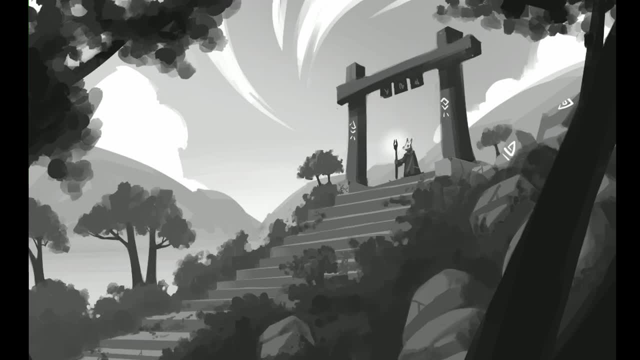 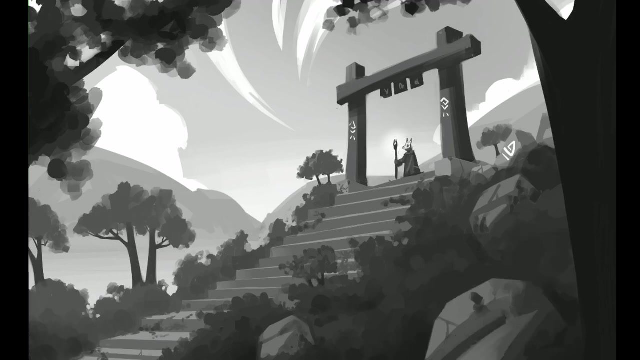 more visible compared to the rest of the painting, where the values are a little bit flatter. Another thing that working with values allows me to do is to really concentrate on the composition, and in this case there are several elements that guide me towards my character and this. 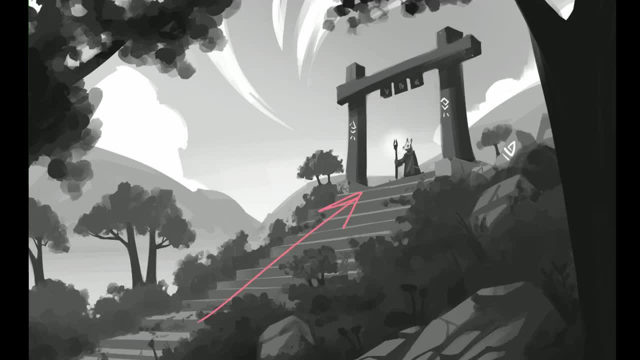 are the stairs that drives my eyes upwards, the swirling clouds that directly point me at the character, the gate that frames the character, and the contrast on the character itself. So this is something to keep an eye on when you're working in values, Everything else. 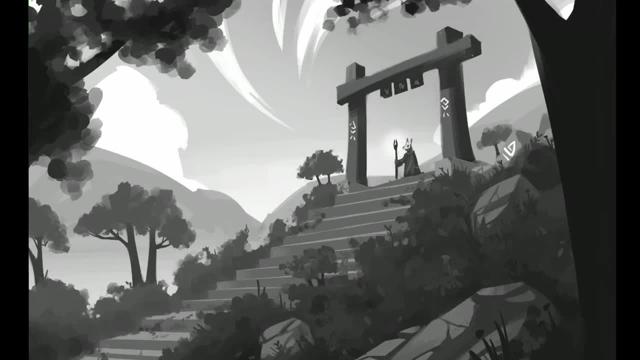 is just adding details to my image and I try to reach a point where I have some indication of light, but I try to keep everything in a sort of ambient light, and this is because when I want to add a more specific lighting, I will do that with color and if you're curious about that, 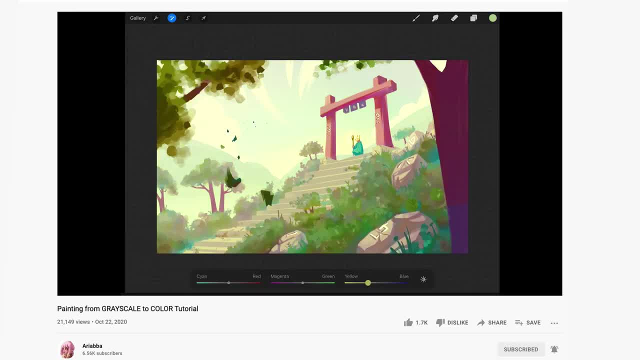 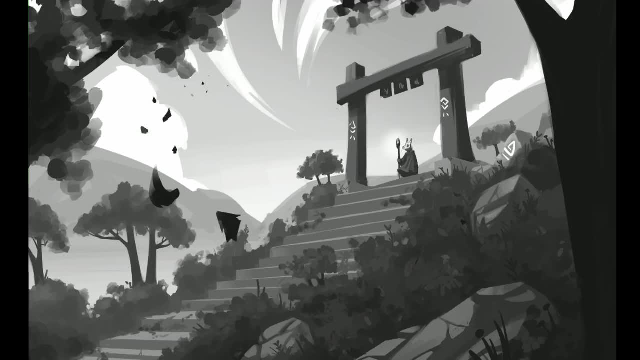 you can watch the sequel of this video where I show how to add color to your grayscale composition. So if you're curious about that, I really recommend to check that out. And this is all for now. so if you're still here, comment below by suggesting the next. 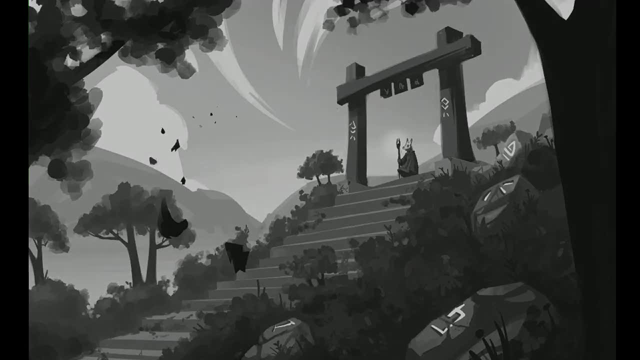 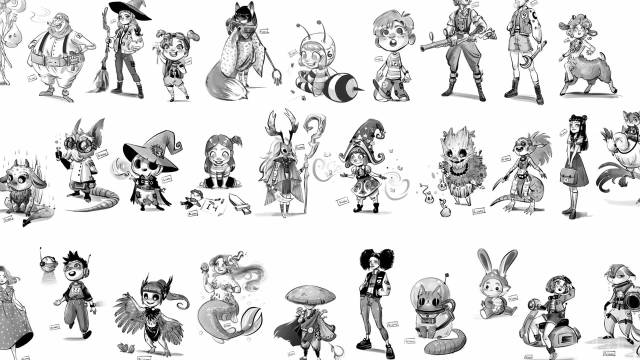 topic you want me to cover and I'll do my best to make it possible. As you all know, I'm always trying to improve and I do so by studying and watching the content of other great artists. I recently tried with a course on a new